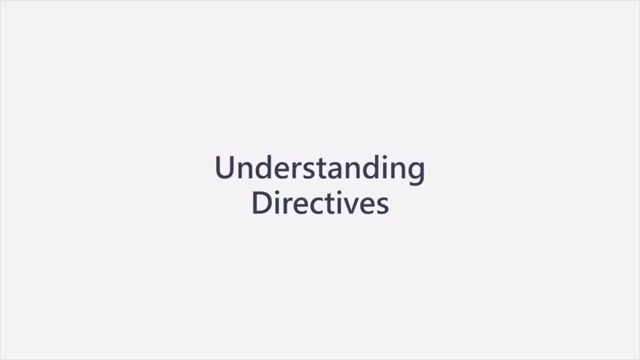 So far in this course, we have learned about Angular components in great detail. We learned that components are the basic building block of any Angular application, And we also learned how to create and use a component. Another key feature of Angular is its directives. 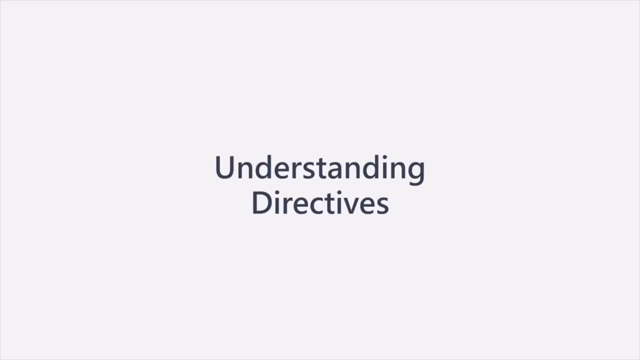 And in this lecture we will learn what is a directive and what is its importance. So, basically, a directive is an instruction to the DOM. In simple words, we use directives to manipulate the DOM. Using directives, we tell Angular how the DOM element should behave. 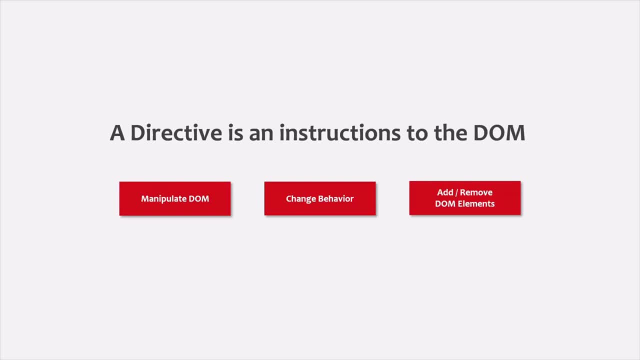 or look like, and also which DOM element to add to the web page and which one to not add. You can change a DOM element's appearance, behavior or layout using directives. They simply help you extend HTML in some way. Directives in Angular can be classified into. 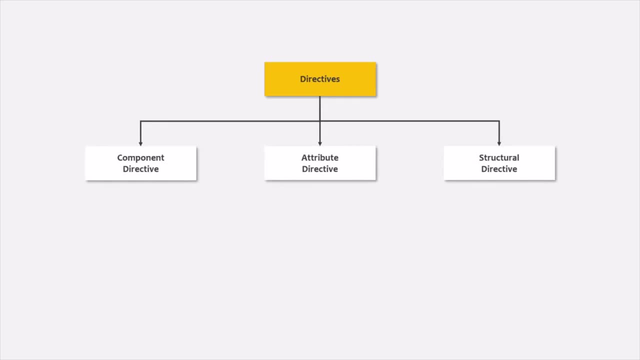 three types: Component directive, attribute directive and structural directive. A component directive is nothing but an Angular component. We learned and used Angular component in our previous lectures, So this component directive is that Angular component. Okay, so component directive is nothing but components in Angular. 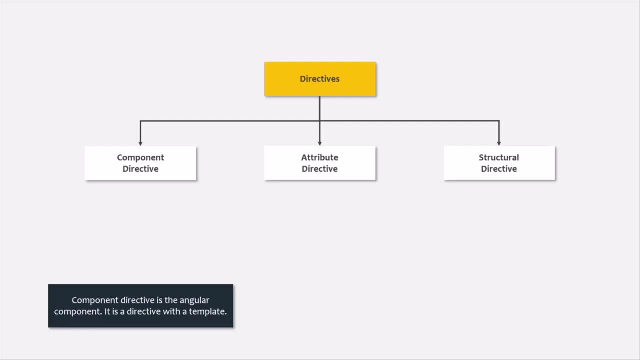 So a component is also a directive, but it is a directive with a template. Components are also a kind of instruction to the DOM. Wherever we use a component there we instruct Angular to render the view template of that component Right. And since we are manipulating, 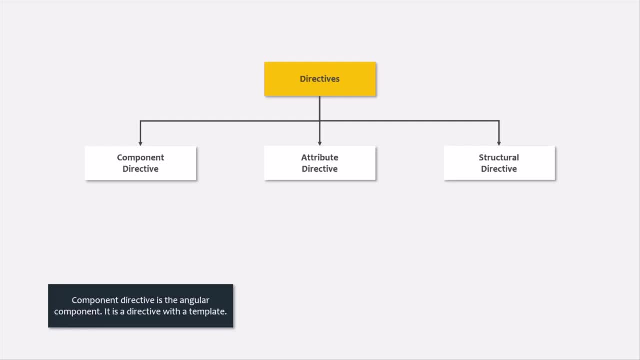 the DOM. when we use a component, we also use a directive to render the view template of that component. But again, it is a directive with a template. Other types of directives do not have a template. So once we place the selector of our component somewhere in the 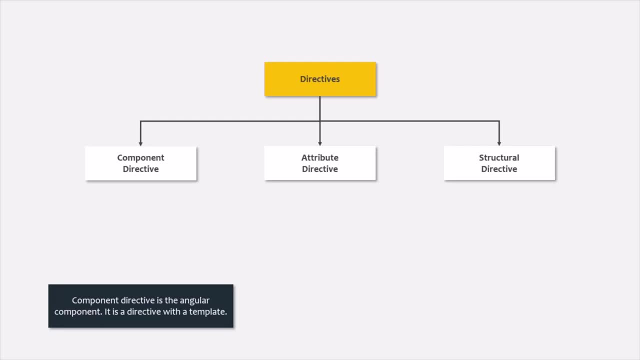 template. at this point of time we are instructing Angular to add the content of our component's view template and the business logic of the TypeScript code in that place where we have used the selector of that component. So this was our instruction to Angular to render the 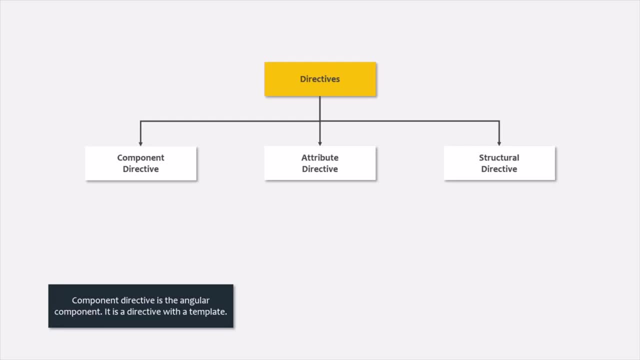 view template of that component. at this point, Components are also directives, but it is a directive with a template. Okay, so keep in mind that components are also directives, but it is a directive with a template. Other types of directives do not have a template. Then attribute directive. 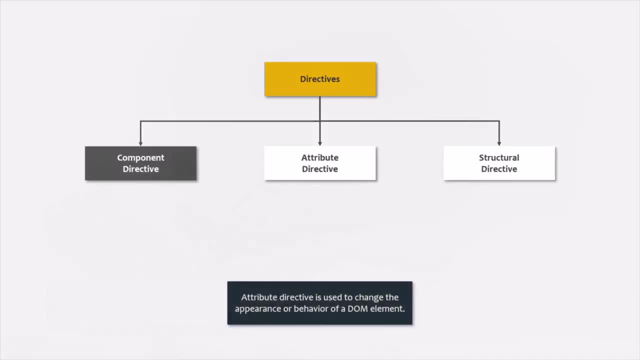 is another type of directive. Using Attribute Directive, we can change the appearance or behavior of a DOM element. Unlike component directive, Attribute Directive does not have a template. It does not render anything on the web page, Neither It removes anything anything from the web page. For example, we can create a custom attribute directive called. 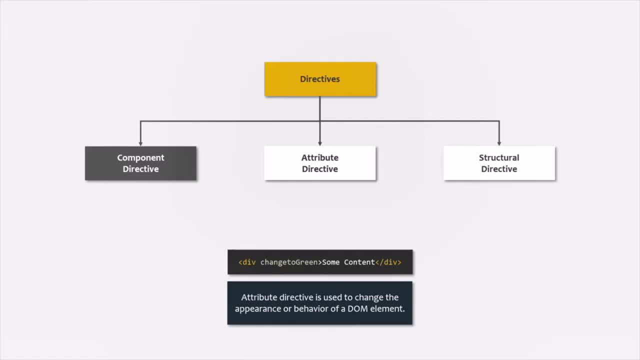 change to green for changing the background color of the web page element to green. So this can be a custom directive which we can build and use it on all those web page elements whose background we want to change to green And, as you can see here we are using that. 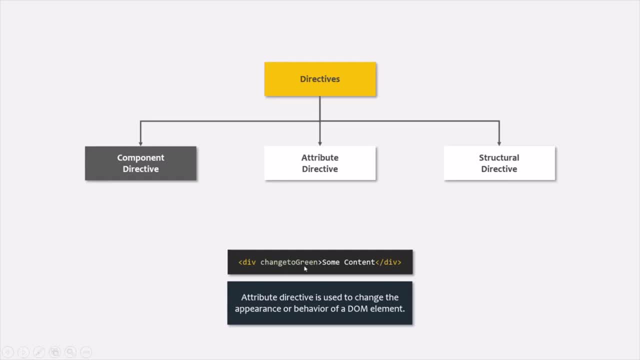 directive like an attribute. Now, since it is an attribute directive, it is only going to change the behavior or look of the HTML element on which we have used it. It is not going to add or remove that element from the web page. We also have built-in attribute directives like ng-style and. 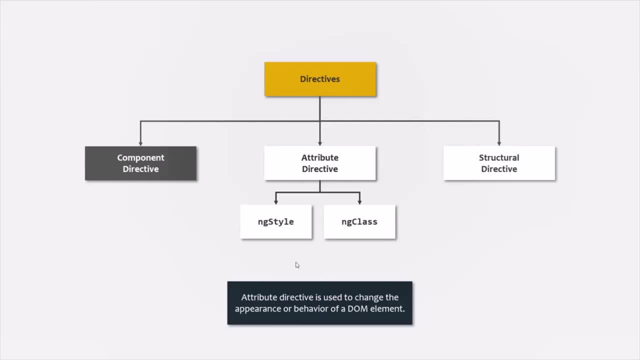 ng-class, which we can use to change the appearance of a web page element. The attribute directives can also be applied conditionally. Now we will learn about ng-style and ng-class built-in attribute directive in our coming lectures. Next we have structural directive. Structural- 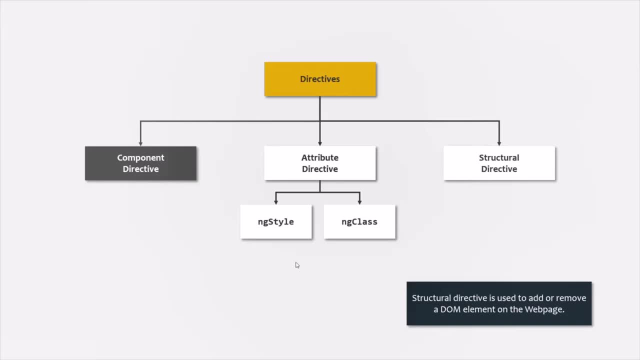 directives can change the DOM layout by adding and removing DOM elements. It basically manipulates the DOM by adding or removing DOM elements from the web page And, just like attribute directive, structural directive also does not have a template. Some of the built-in structural 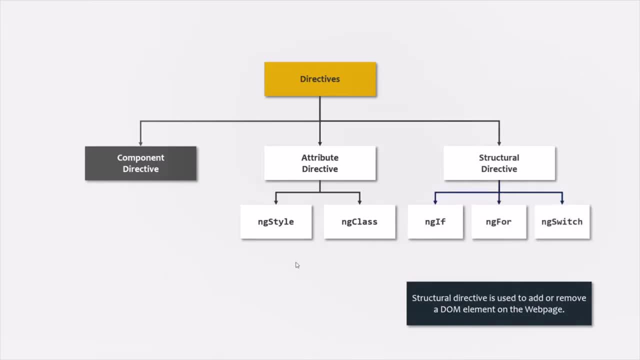 directives available in Angular are ng-if, ng-for and ng-switch. Now, one important thing to keep in mind here is that whenever we use a structural directive before that structural directive, we use an asterisk, For example here on this development, when we are using this ng-if directive before that. 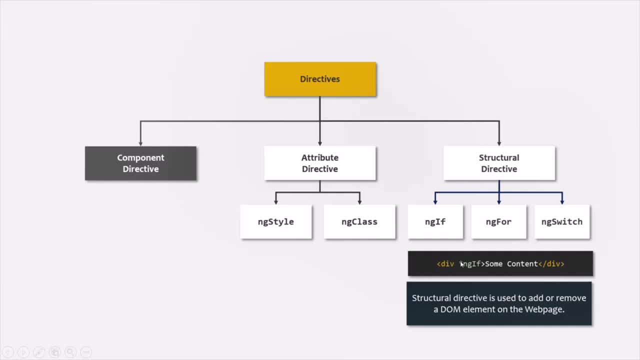 directive, we are using an asterisk. This simply tells Angular that the directive which we are using here it is a structural directive. It is going to manipulate the DOM by adding or removing DOM elements. Again, we will talk about structural directive and these built-in. 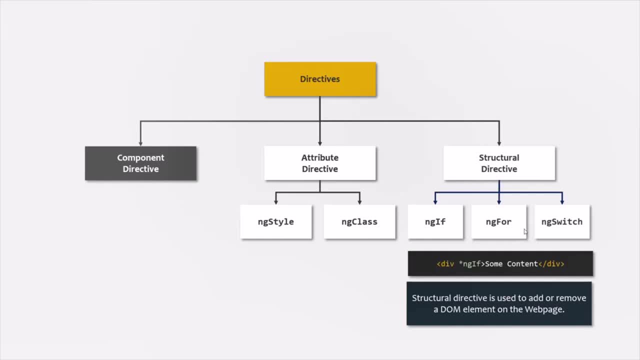 structural directives in great detail in our coming lectures. Now we typically add directives with attribute selector, but technically the same directive will always be used. So we will talk about thoseructional directives in a moment. supporters: selector, but technically the selector of a directive can be configured like the selector of a component. So we have